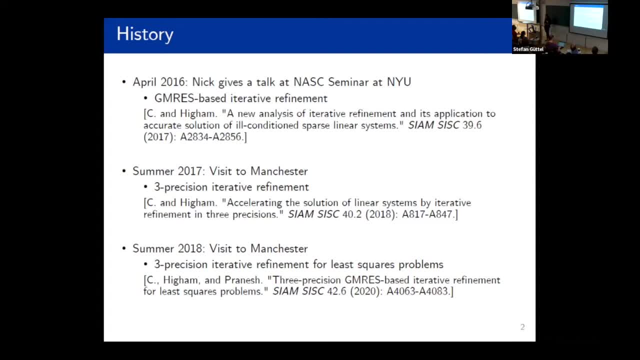 scientific computing seminar on multivalued matrix functions, And so, as is tradition, we take the speaker out to lunch afterwards, and so I was lucky enough to be sitting close to Nick, and he mentioned to me at some point I have some problem with GM res. I wonder if we can talk about it, And 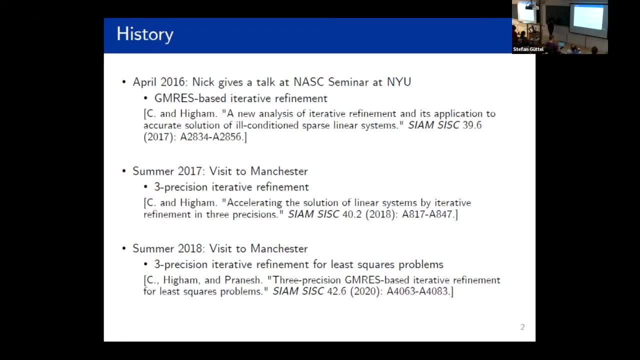 so Nick stopped by my office after lunch and he told me this idea of iterative refinement and maybe we can use these, And so I said: okay, okay. And so you know, then Nick went back to Manchester and, like Dennis said, 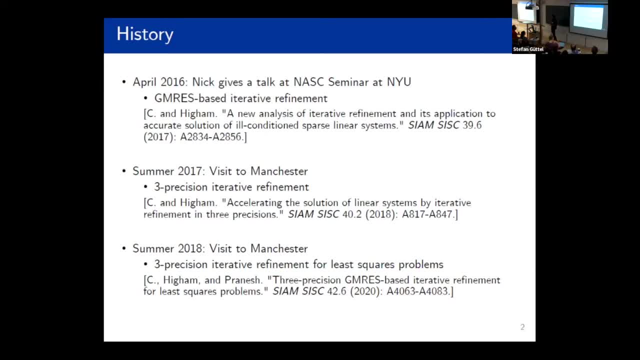 you don't want to disappoint Nick, I am. so I set to work on this And a little while later emailed some results to Nick- And again he was very courteous because I'm sure these initial results I sent him was just terrible. But we iterated on this and refined it And over the 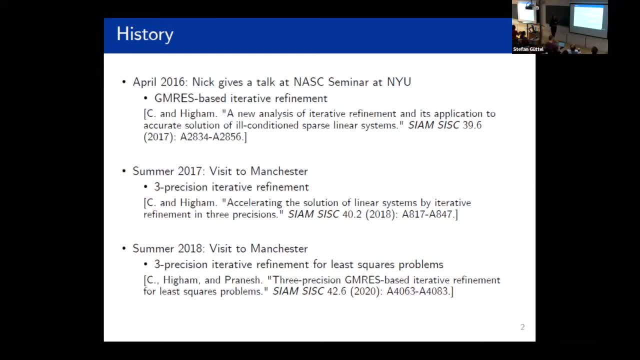 course of that year, we refined it, And so I said, okay, I'm going to do this. And he said I'll work on this. And he said, Okay, here's what I'm going to do, And I think this is gonna help. 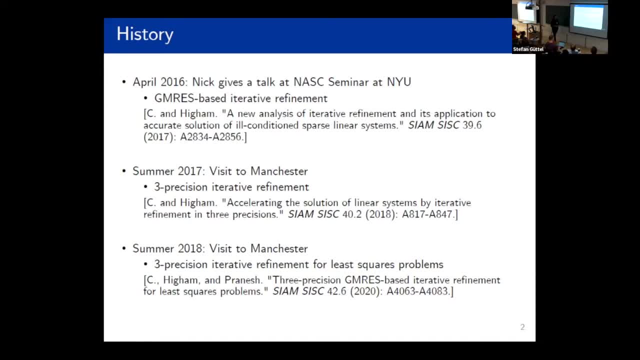 me to kind of work on this. That's how it all came together, And so we did this over the course of about 60 hours And we talked about this, this first paper together on GM res based iterative refinement. Okay, so then, around that time, so in 2017, was right when, in video, I come out with 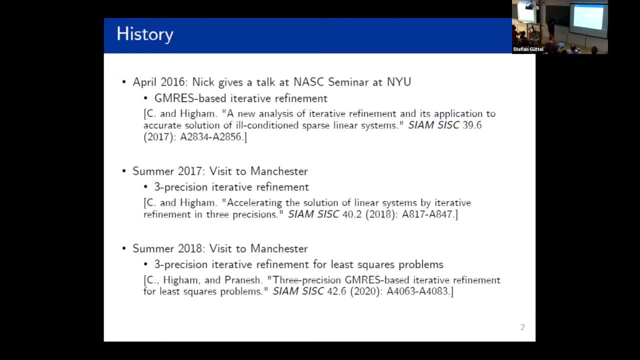 this V 100 GPU that had these half precision tensor cores, And so I don't remember the exact timing, But Nick was at a, had a meeting with Siam in Philadelphia and made a stop over in in New York, and has we had a brief meeting together and he he mentioned to me, you know, I think we could do. 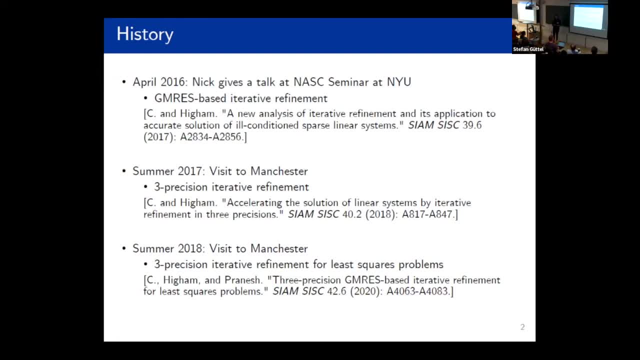 this in three precisions. you know why not? And I remember saying, Hey, I think we could do this in three, why not? And I remember him saying to me: I think that this could have really big impact, And so for me, this is my most highly cited paper that came out of that brief discussion with Nick. So 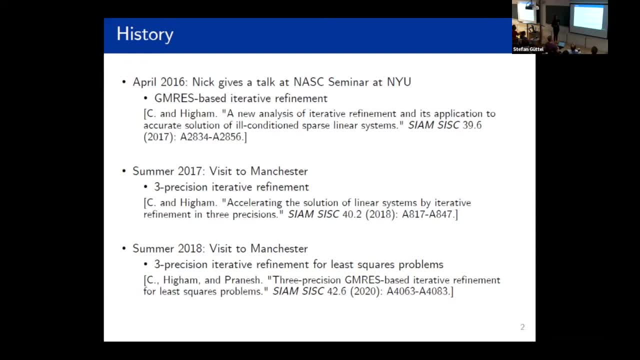 thank you very much, Nick, for that. He invited me that summer to visit Manchester, And so we finished the work on the three precision iterative refinement paper. I also visited here the subsequent summer and we worked on applying this to least squares problems, And that paper took a. 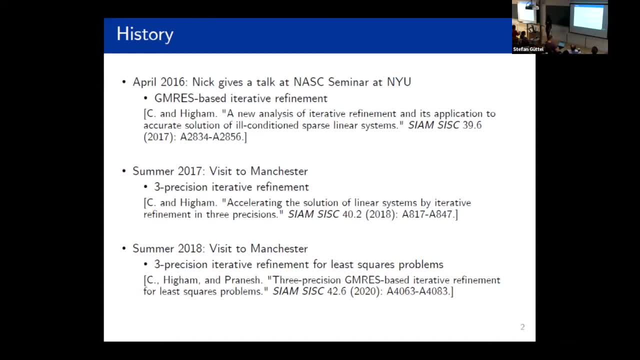 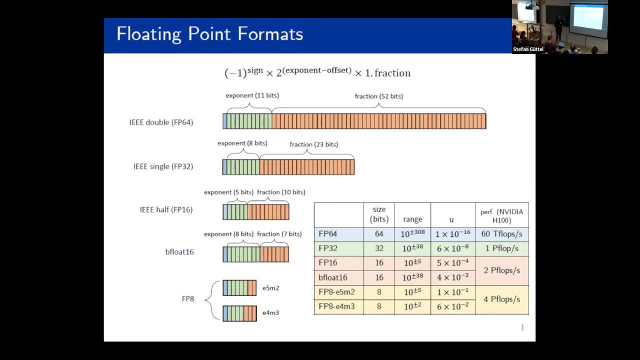 little longer, but that was my own delay. Okay, So my talk again will be based on mixed precision, And so we all know and love double and single. You know, when I started working with Nick, this FP16 and BFloat16 formats had just started to come out, And now just 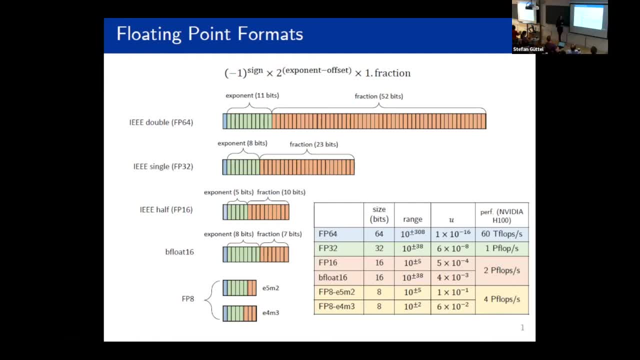 earlier this year. now the NVIDIA has a GPU with even quarter precision And there's two different variants depending on you can put one more bit in the Mantissa or not. Okay, And so here is just a table. So here's the double precision, single precision. 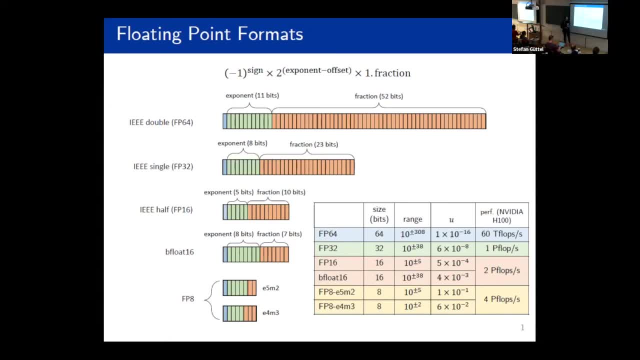 the 16-bit formats and the 8-bit formats And you can see here the advantage. So this is kind of the best performance you could hope for on the latest NVIDIA H100 GPUs And so you can see there's a clear benefit. right, We can get much better performance if we can make use of 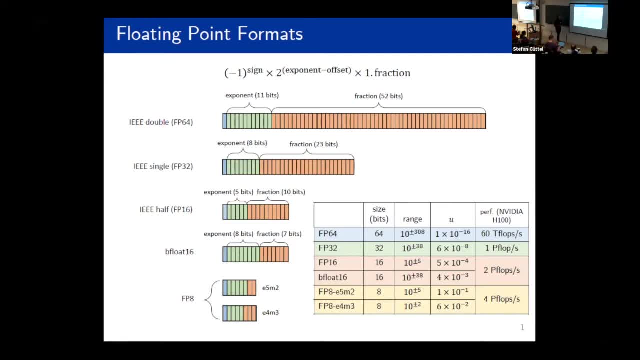 these low precision formats. Okay, The trade-off is right. we have less precision, right, So this? U will be the unit roundoff, And so we can get much better performance if we can make use of these low precision formats. Okay, The trade-off is right. we have less precision, right, So this? 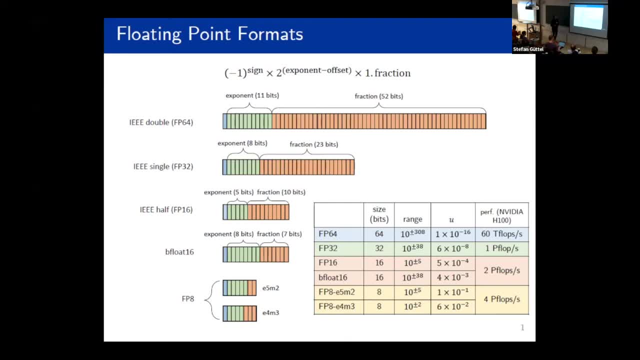 U will be the unit roundoff, And so we can get much better performance if we can make use of throughout my talk, And we have a smaller range of representable numbers. So which of these formats is most appropriate for you to use will depend entirely on the data you have and how much. 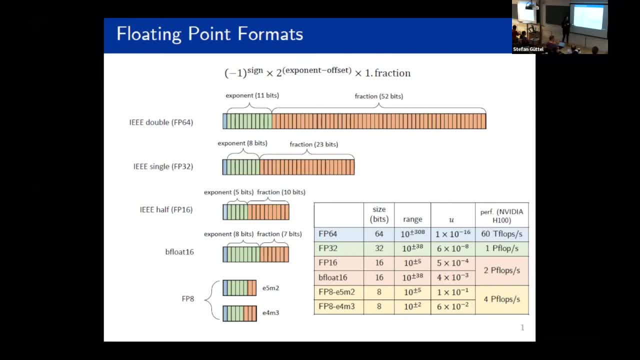 precision accuracy you need, Okay. So if we take a nice small number like 60,, for example, okay, that falls nicely into the range of all these formats here, Although if you use this E5M2 format, the 60 unfortunately gets rounded up to 64. 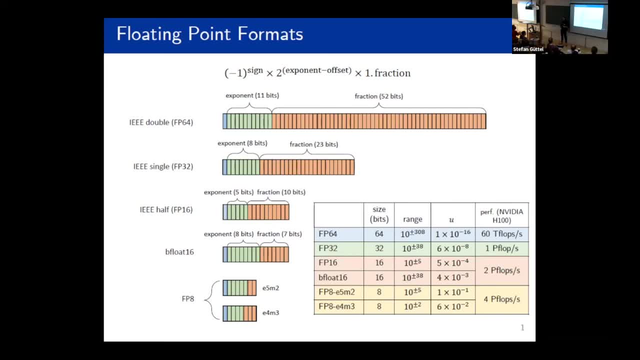 Okay, But if you use stochastic rounding you might get lucky, and it's only 56. So if you try and use fewer bits than that, it might overflow to infinity. So we're not going to go there. Okay, And so there's a long history of using mixed precision in numerical linear algebra. 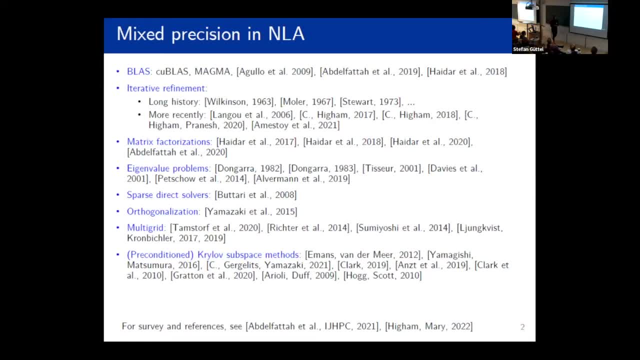 In iterative refinement. this goes back to Wilkinson in the 60s, And Gerard Morant recently pointed out to me that Doolittle was even doing this much earlier than that. Okay, And so there's been a lot of work in developing BLAs that exploit these. Okay, So if you use stochastic rounding, 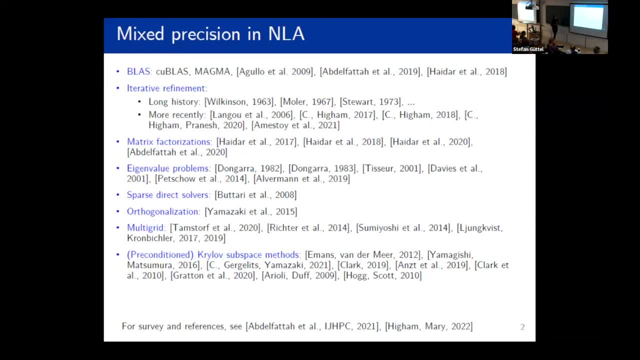 these tensor cores, iterative refinement, like I said, for both linear systems and least squares problems, matrix factorizations, eigenvalue problems, both dense and sparse, sparse direct solvers, orthogonalization, multi-grid and iterative methods. And so there's a couple. 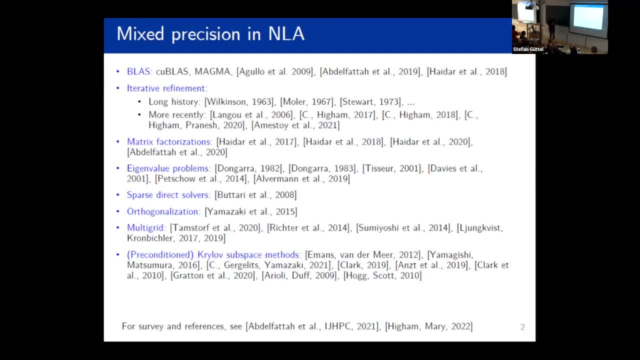 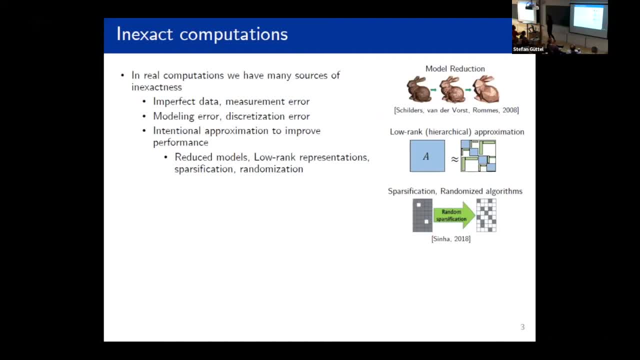 in the scientific computing or data science world, we don't just worry about floating point arithmetic. In fact, people often just kind of ignore that because we're dealing with so many other errors that are usually of much greater magnitude. Okay, So just to start off with 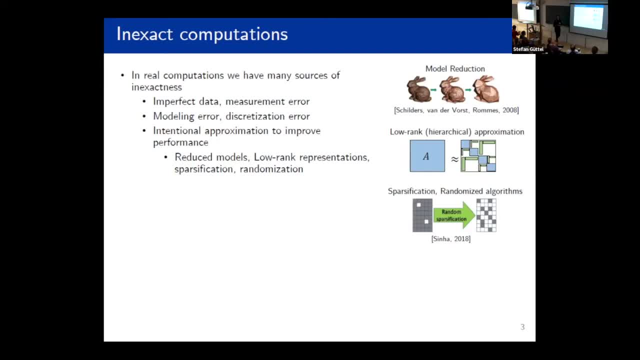 we're working with imperfect data. Okay, We have a precision with which we can measure the data that's going into our matrix. our right-hand sides- We have modeling error, discretization error And, a lot of the times, we're usually making some intentional approximation at the algorithm level in order. 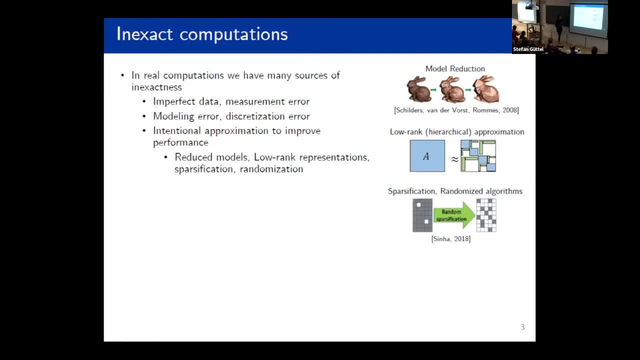 to get better performance or to reduce the memory and things like that. Okay, So there's just some examples of that: our model order reduction using low rank or hierarchical approximations, or doing some kind of sparsification, or using and or using randomization. Okay, And so you might. 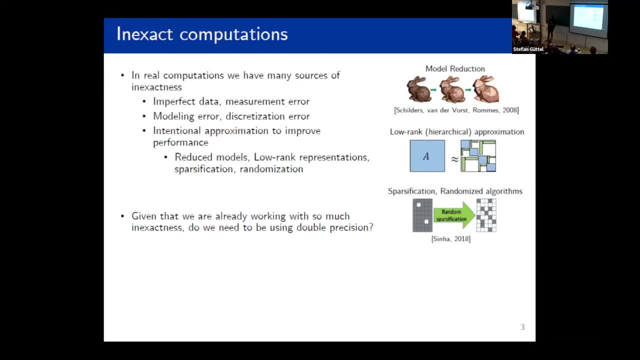 ask: okay, so, given that you're already working with so much inexactness, do I really need to be using double precision for all my computations? And the answer, I think, is usually no in a lot of cases. Okay, And so I will steal this analogy that I've heard from 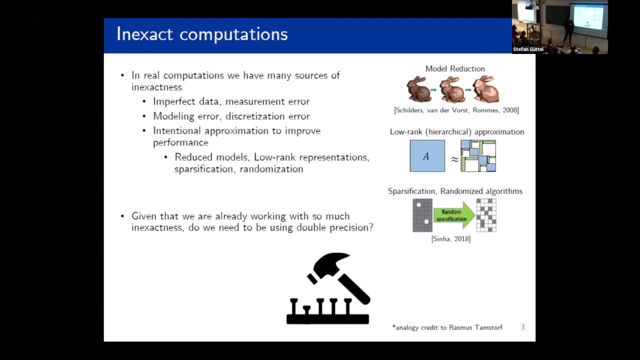 Rasmus Tamstorf, where, if I think of these nails as my errors right, there's no point in hammering down the finite precision error so small when I have all these other nails still sticking up. Okay, So I like this analogy. It captures it very simply. I will point out that it can be. 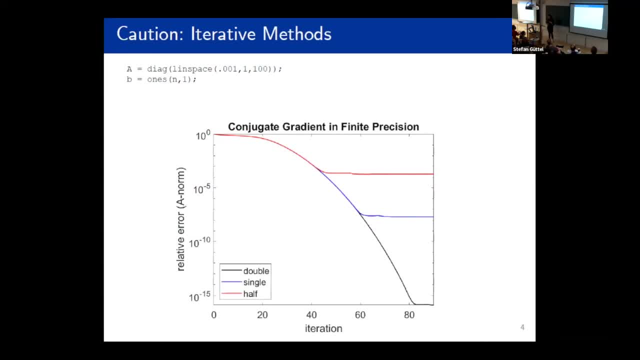 more complicated than that? Okay, And so here's one example that I know of that's dear to me, Where things can be a little more complicated. All right, So if we look at just running the conjugate gradient algorithm in finite precision, Okay, So I have a very simple matrix here, So my 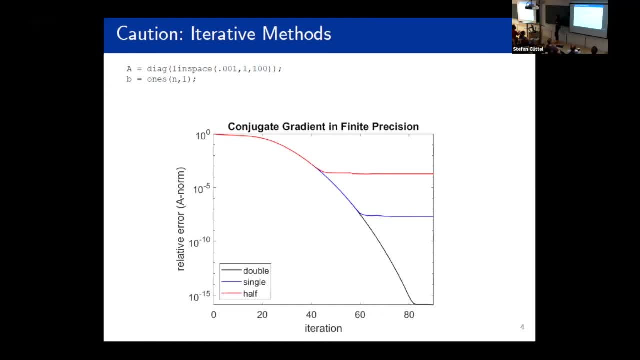 matrix is just a diagonal matrix, condition number 1,000 with equally spaced eigenvalues. Okay, My right-hand side is just a vector of ones, Very simple, Okay. So here I'm plotting the iteration on the x-axis and the relative error in the A norm on the y-axis, with double precision in black. 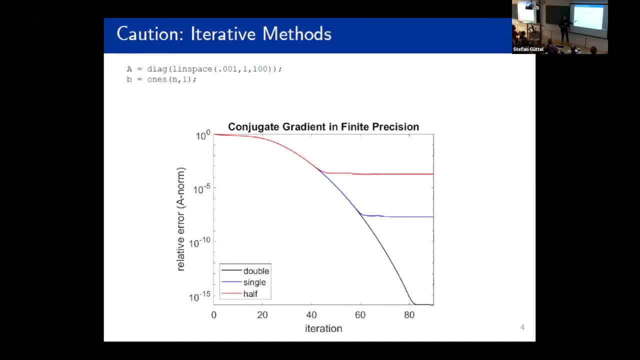 blue in single and red: Okay. And so if you look at this you say, oh, okay, my other nails are, you know, much higher. here I can get away with using half precision. here I only need 10 to the minus 4, 10 to the. 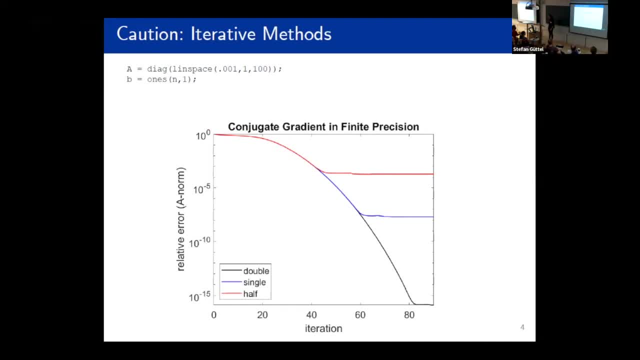 minus 3.. That's fine, I could run CG in half precision and lose nothing, Okay, But this is not always the case. Okay, So here is a matrix: same condition number, same largest and smallest eigenvalues, but the distribution of eigenvalues is different, Okay, So here I won't say they're. 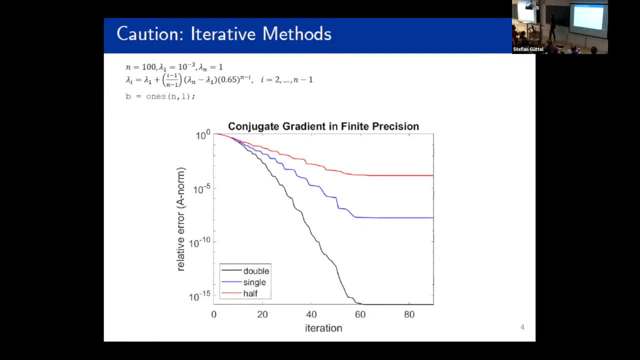 clustered, but they're accumulated towards the left side of the spectrum so that I have large outlying eigenvalues. And this is actually a known case where CG is more subject to the effects of finite precision error when there are large outlying eigenvalues. Okay, So in this case, 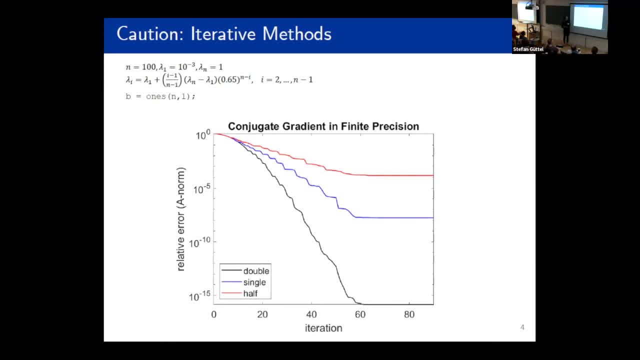 you know, I'm not just losing accuracy. The accuracy might be fine, but I'm also converging much slower when I use lower precision, Okay, And so that can kind of, you know, detract from some of the performance benefits that I might see if I have to do many, many more iterations. Okay, So we. 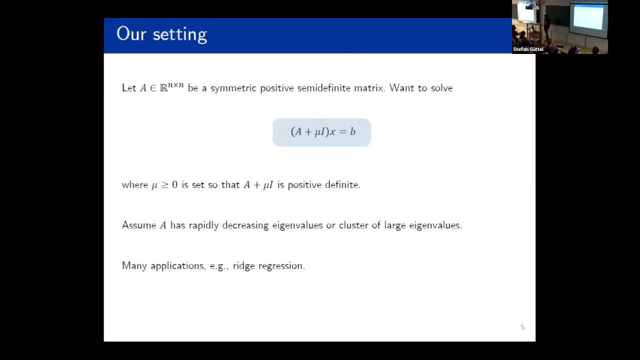 hammer our nails down, but we have to be careful doing so. Okay, So I'll talk about some recent work of mine today, And so this is a joint work with my postdoc, Ieva Dauzhitskaita, And so in 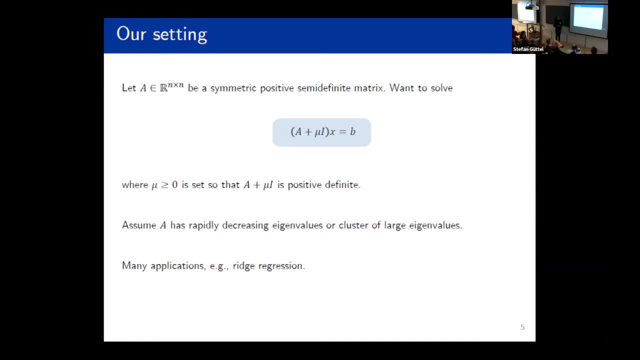 our setting, all right. so we want to solve systems of this form. So I have a square matrix, A, It's symmetric, positive, semi-definite- Okay, I have some shift parameter here And so this will make A plus mu I positive definite. Okay, And I'm going to assume in our desired case A is going to have. 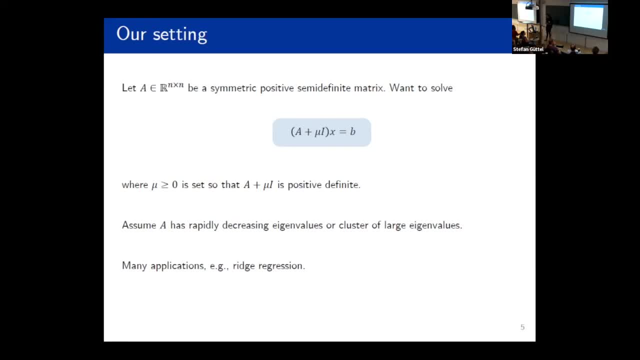 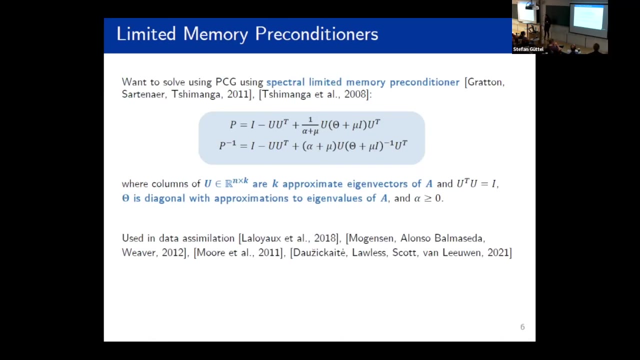 two eigenvalues, which is either some- And so this comes up in many applications, So regularized least squares, for example in ridge regression. Okay, And so I want to solve this system using the precondition conjugate gradient method, and I'm going to use preconditioner And I'm going to use a spectral limited memory. 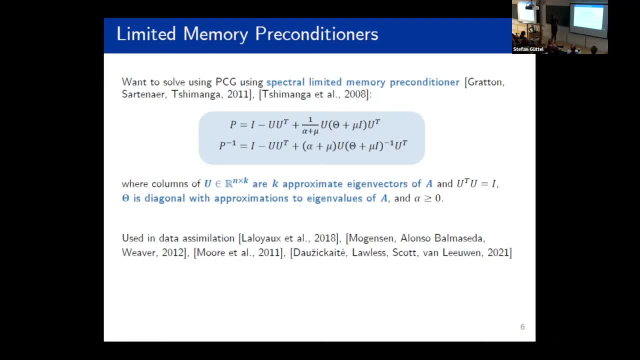 preconditioner, And so there's a lot of work on this. So my matrix, where's the oh? okay, So my conditioner P has this form. I can also write out its inverse, okay, And so U here. so this is an. 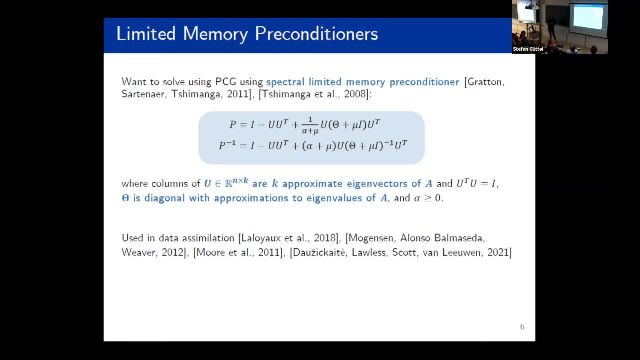 n by k matrix, whose columns contain approximate eigenvectors of A and they're orthogonal, And so my theta here is diagonal, that has approximations to the eigenvalues of A. okay, So this comes up in data assimilation, which Jennifer and others have done a lot of work in. 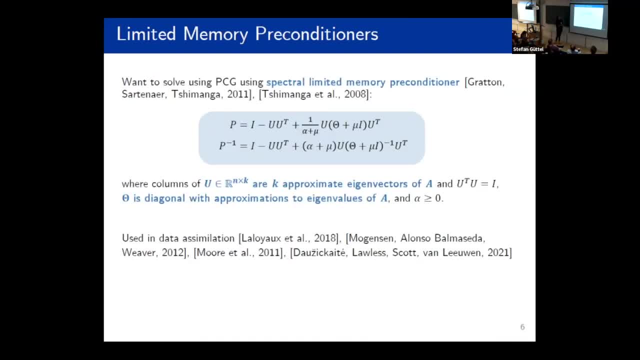 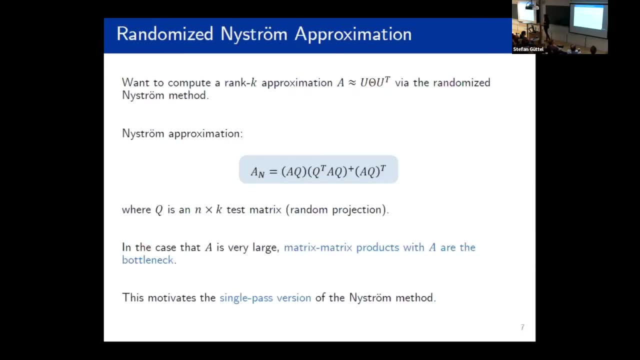 Okay, and so what do I need to do? I need to in order to construct my free conditioner. I need these approximate eigenvectors and approximate eigenvalues. okay, So I'm going to obtain them using a randomized Nystrom approximation. So I want to compute some rank k approximation. 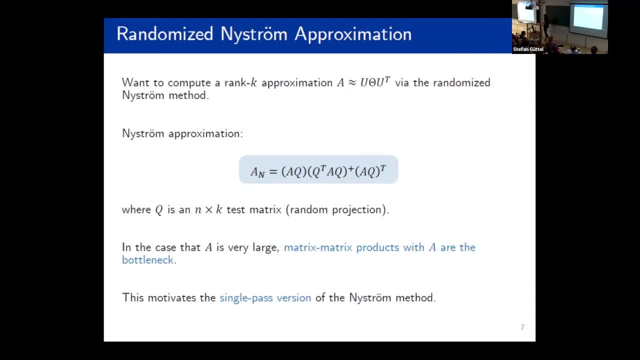 using the Nystrom method. okay, And so my Nystrom approximation takes this form here, and so Q is my test matrix. We're going to use a random projection And in the case that so you could pick Q to be based on the columns of A somehow, because the quality of this 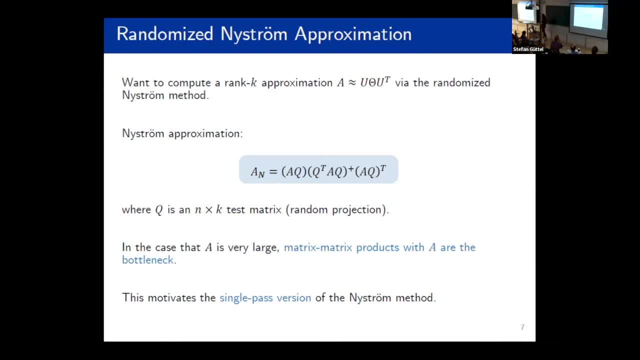 approximation is going to depend on on the range of Q. So in the case that A is very large, we're just going to use Q as just a random orthogonal matrix, And so I want to avoid matrix-matrix products with A. So I'm kind of 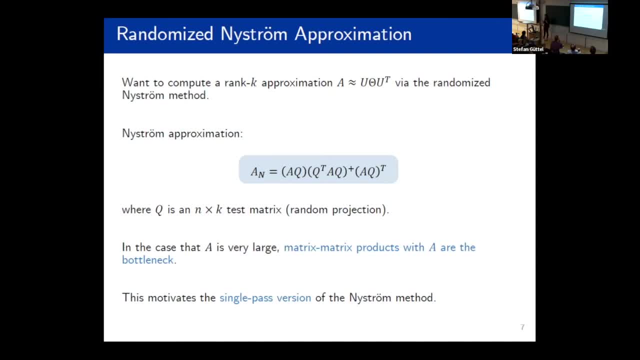 assuming that doing A times something is the bottleneck in my code, So we're in the setting where A is very, very big, Okay, and so here is how this works, And so this algorithm is from TROP and others, So this is a stabilized version of this. 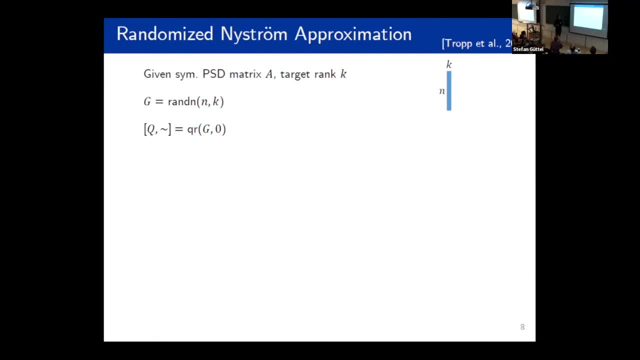 Okay, so first I'll generate a random Gaussian matrix. You don't have to use a Gaussian- You could do something more structured if you wanted to- but I'm just assuming a Gaussian here. Okay, I will take its QR factorization. Okay, and then here I'm going to do: Y is A times Q, So 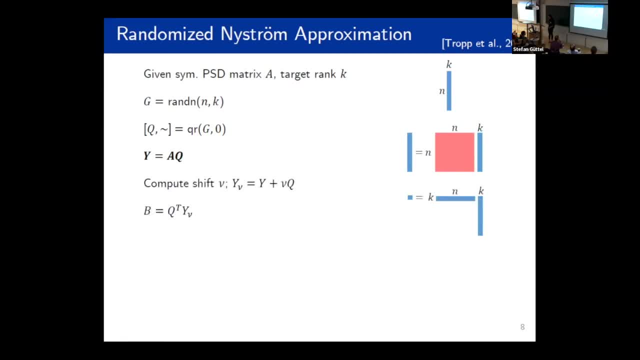 that's my expensive part here. That's the big matrix times, some vectors. Okay, I'll compute some shift to this Y. I'll do Q transpose times Y and I'll get this tiny matrix B. Okay, I'll do Q solve for the eigenvalues with my cool math, excuse me, but trying to make sure. 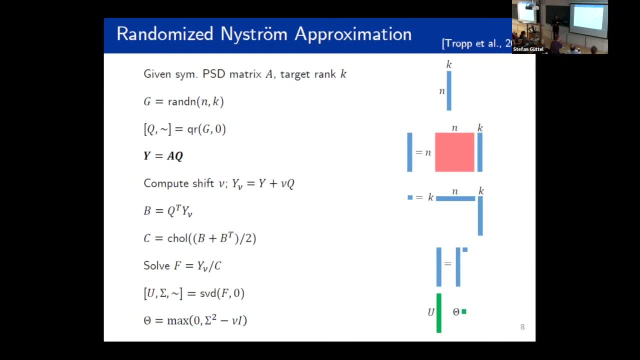 the Cholesky doesn't fail en me to get this Cholesky factor. I will solve on the right and then I can get. I'll do the SVD of the result and I can get out my U, which is what I want. 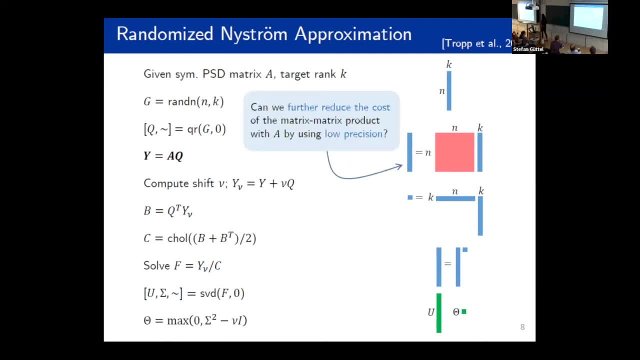 and then the singular values and I'll undue the shift that I did and then I can construct the eigenvalues. Okay, so the question is: given that this is the most expensive cost here, right, doing this matrix times these vectors, that in lower precision? okay, and so again, here are my, here are my two nails here. okay, so i can. 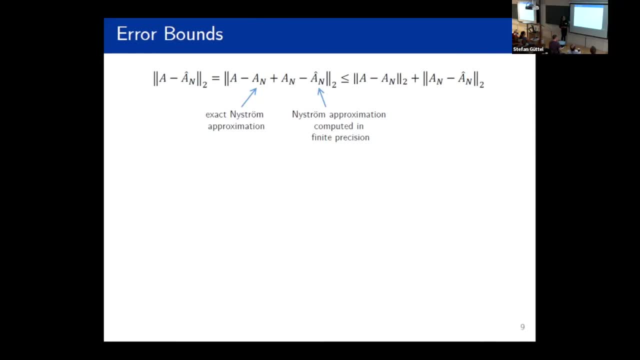 i can write, uh, the total approximation error as the the sum of these two errors. so this, a sub n is going to be the nystrom approximation, if i computed everything in exact arithmetic, okay, and the a? n with a hat is going to be what i actually get when i do it in finite precision. 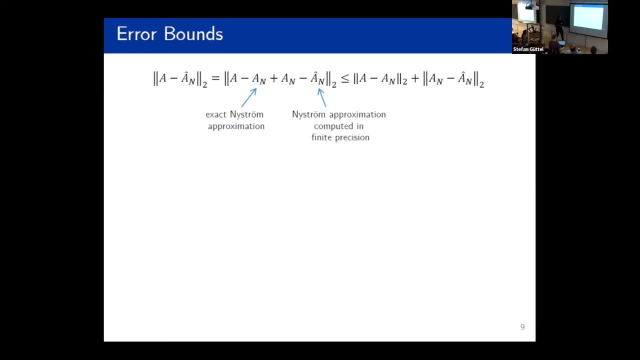 okay, and so usually i'm, i'm, you know, if i don't want a very, if i want a pretty low rank approximation, you know this, this error here, well, this exact approximation error, will be pretty large, and so i can hammer down my finite precision error to to match that. okay, and so there are. 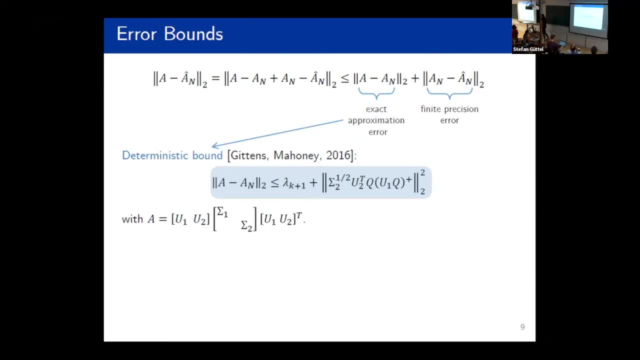 existing results on the exact approximation error. so a deterministic gap bound was given by gittinson mahoney, um, and that could be that could be pessimistic. there's also an expected value bound, um that's given. okay, all right, so our goal, so someone, someone's already done the 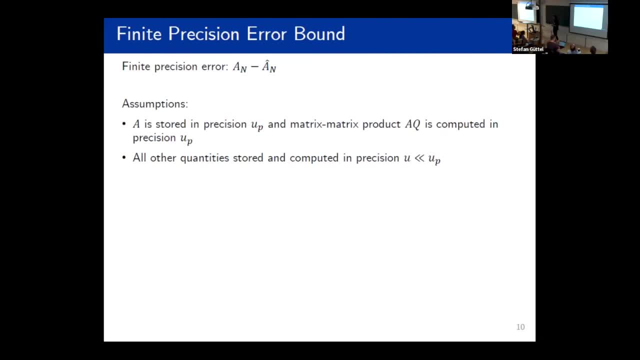 you know the exact, you know the exact, the exact error. we want to look at the finite precision error. okay, so again, my finite precision error is the difference between the exact nystrom approximation and the one computed in finite precision. okay, i'm going to make the simplifying assumption to start off with: um, that i, i'm that. 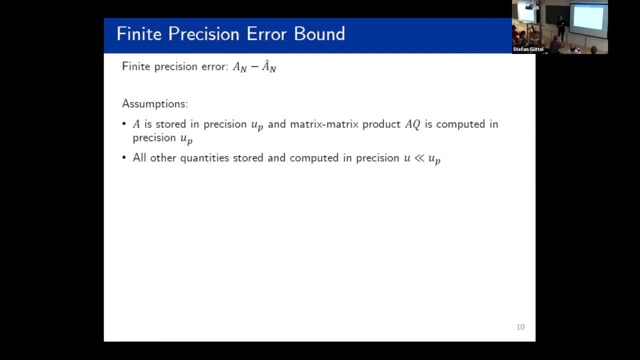 this is the only part i'm doing. let's say, in exactly, is the matrix, matrix, matrix, product a times q, all right, and i'm going to do that in some precision called up right. everything else is done in a working precision which i'm going to assume is much smaller. we could get away. 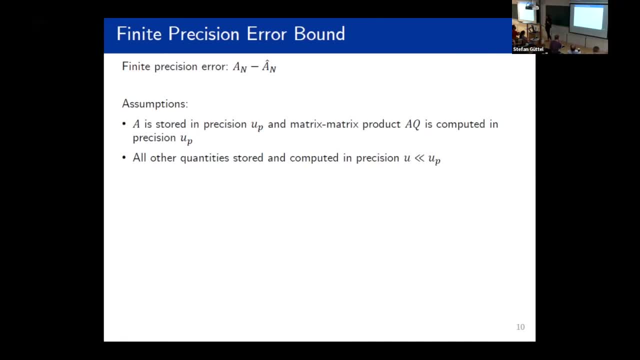 with we could. we could do away with that and um, but it would just complicate the analysis, okay, and so i, you know, you do a couple pages of of analysis. i won't bore you with that, but we can write down a bound of this form, okay, so the difference between the exact nystrom approximation and the finite. 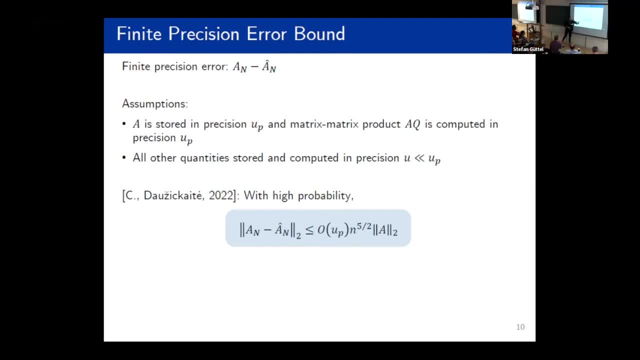 precision. one okay is bounded, as you know, some factor of the precision with which i'm storing the matrix and computing this matrix, matrix, product, um, some dimensional constant which is much larger than than you actually see in practice, very worst case. and then some norm of a okay, and so, if okay, so i'm gonna, i'm gonna fudge the. 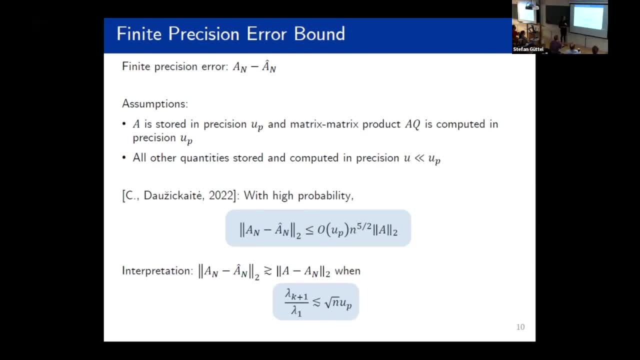 dimensional constant, because we really don't see end of the five halves in practice. so what is my interpretation? so what does that mean? so i want to know, you know, when is my finite precision error going to get b, b larger, grow larger than the exact approximation error? and i can say that that will. 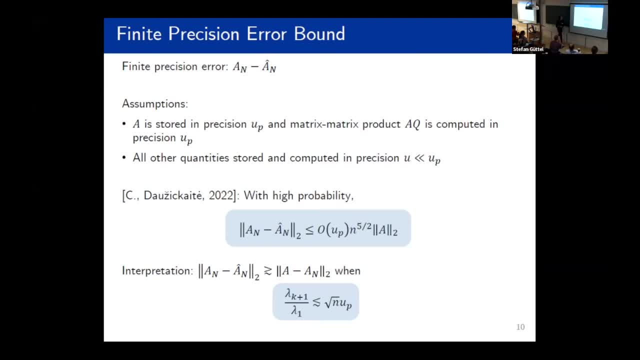 happen, uh, when this, this ratio, uh, this, this k plus first eigenvalue, divided by the largest eigenvalue is, uh, you know, around n squared of n times up. all right, so this kind of gives me, if i, if i, you know, know something about the, the gaps in my eigenvalues, i can kind of figure out, okay, what, what is my, what precision can i use? 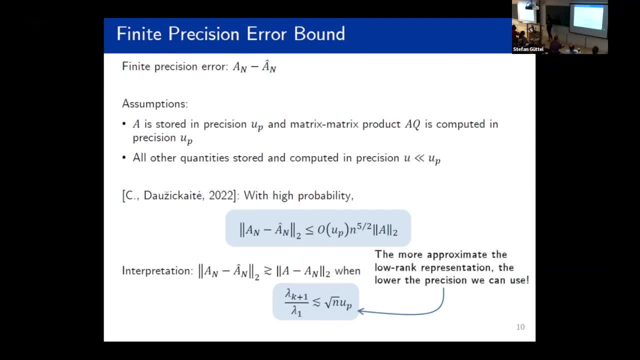 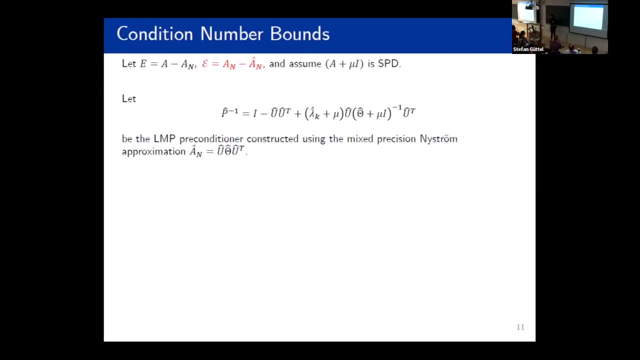 here and get away with all right and intuitively. the the more approximate, the lower the lower rank representation we want, the lower the precision we can use. okay, okay, so now, like i said, we want to use this as a preconditioner, uh, in the conjugate gradient method. okay, so how good of a preconditioner. 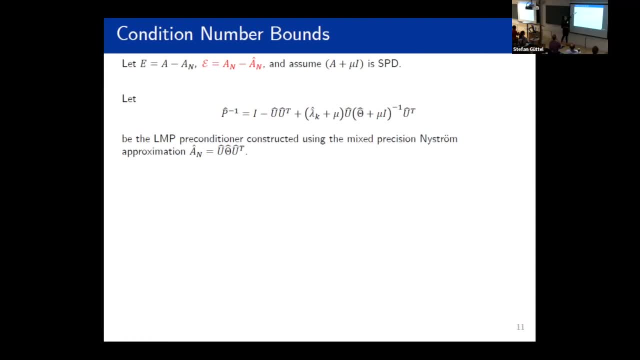 is it going to be all right? um, so i'm going to define two quantities here. so this e is uh. so just just to simplify this, so i don't have uh, you know, so it fits on one slide. i'm going to call the exact approximation error e and the finite precision error is curly e. okay, all right. so here's my limited memory. 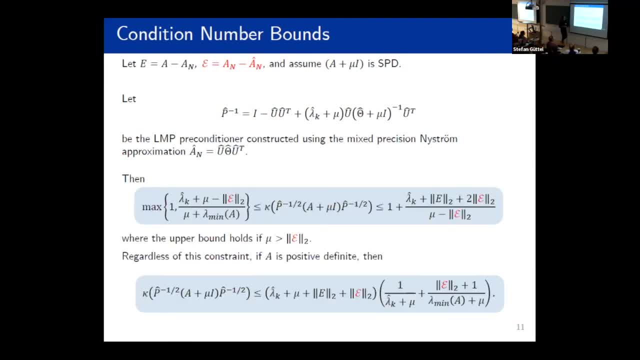 preconditioner. so how good is it all right. so i i will again stress that, as i just showed in the previous slides, condition number does not tell you the whole story about cg. but you can say: if the condition number is small, then you will converge quickly, okay. 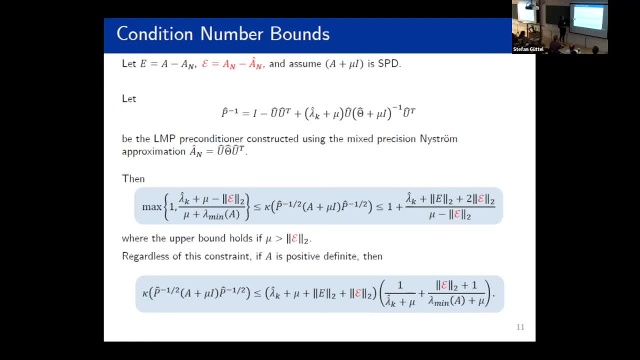 all right, so then we have these, these bounds. okay, so this first expression gives me a lower and an upper bound. of course, this only holds if this mu is is greater than my finite precision error, otherwise this falls apart. and in the case that a is positive, definite, then i have another upper bound which also holds. okay, so these 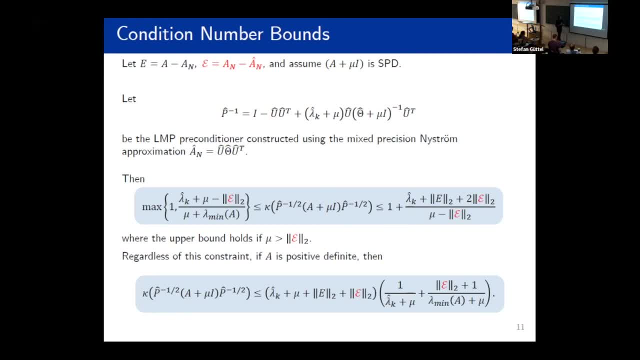 these red quantities- here are the ones that show up now, because we've taken finite precision error into account. okay, and if you set that to zero, then it reduces to the bounds that have already been proved for the exact case expression. you can see, i'm going to use the equation of cg as a preconditioner. 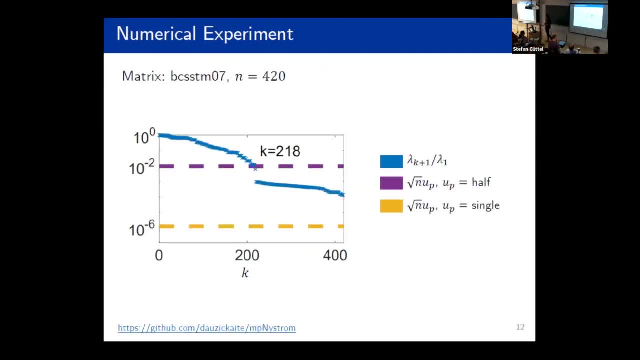 case in the literature. All right, so let me just show you a numerical example of how this works. So this is a matrix from the sweet, sparse collection. These are just small problems. You can find our code for running this here. Okay, and so here. this is just to give us some intuition. What can 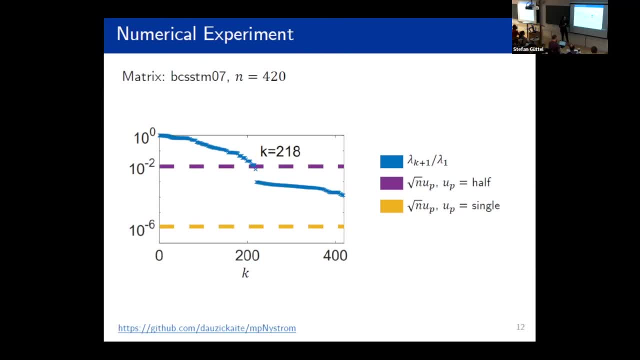 I expect to work Okay. so here's the value of k. right, That's the rank, let's say the rank of the knee-storm approximation I'm taking. Okay, here I'm plotting, these are just kind of scaled. 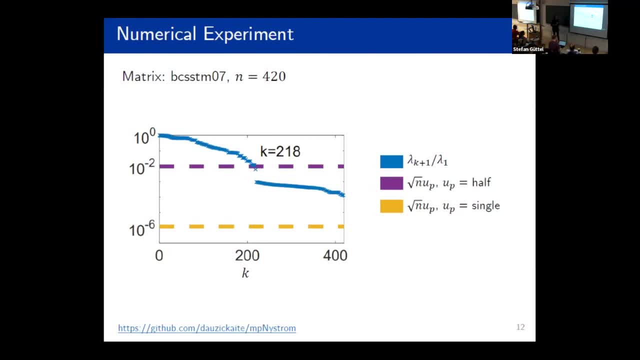 the normalized singular values, so k plus one over the largest one, All right, and here's square root of n, up for half, and here's square root of n, up for single. Okay, and so what we can intuit is that you know where this crosses. that's about when I'll start to see the finite. 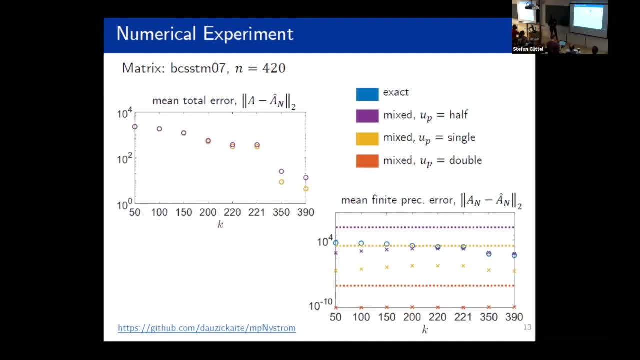 precision error dominate, Okay, and so if we look at that, that's the case, All right. so here, blue is exact, Okay, purple is using half, yellow is using single and orange is using double. And so you know, you do see around, you know 200 to 220.. That's. 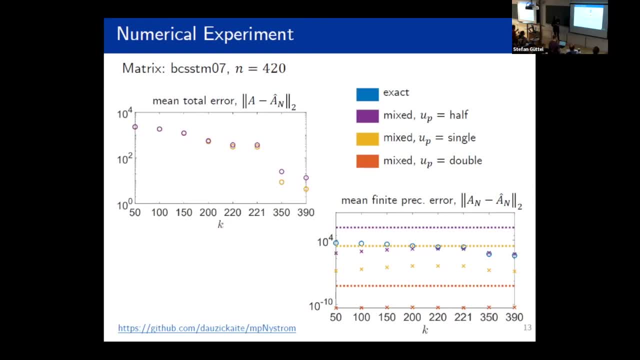 where the half precision starts to. you know, give me a deviate, let's say, and you can see the effects of using the lower precision. Okay, but for a single, you know, fine, you could use that, no problem at all. Okay, and now we have the also the mean finite precision error Again. 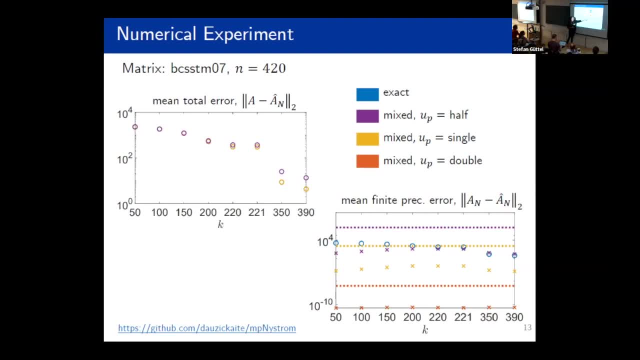 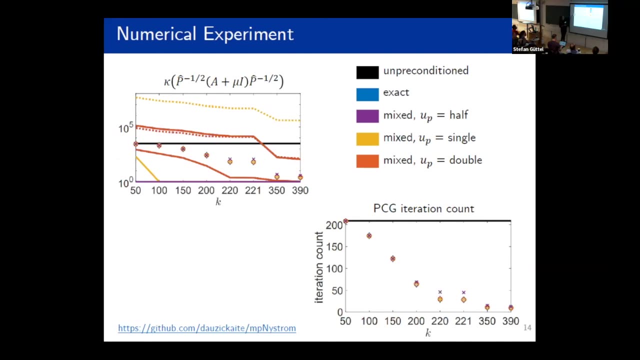 these. so these are the actual measured quantities and these are the bounds. So the bounds are, you know, given a pretty big overestimate in most cases. Okay, and so what about its use as a preconditioner? Okay, so here I have, I'm plotting the 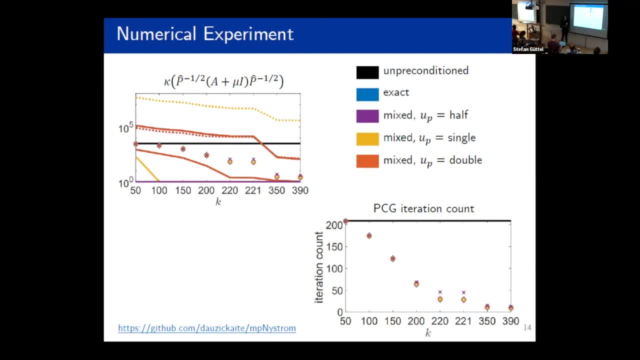 condition number. All right, so the markers show the actual measured quantity and kind of the lines are giving the upper and lower bounds. Okay, and so here we have. we can see that again, around, you know, 200 to 220, around 218, that's where you know we see a deviate. 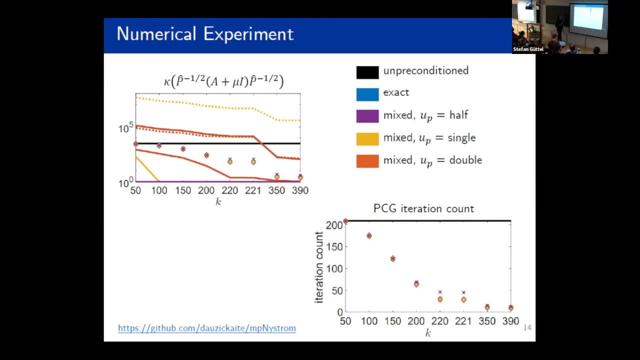 and so we're looking at the variation of using half precision, which is predicted by our heuristic. you know the bounds, however, for half precision, especially the lower bound, are kind of useless in this case. Okay, and what about the number of iterations that we actually see in the precondition? 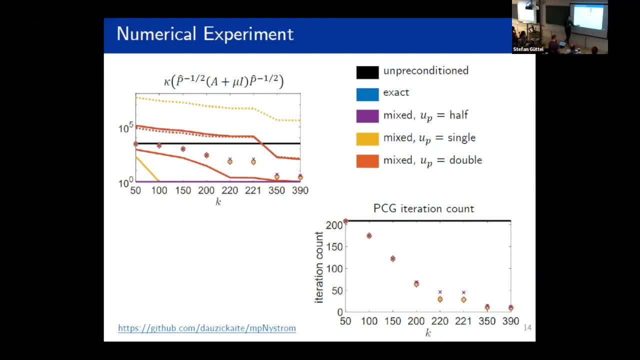 conjugate gradient method Again, until we need a you know rank around 218,, 220, we really don't see much effect at all of using half precision, so we can totally get away with it, okay. and so just just to just say, we did try some things in quarter precision, um. 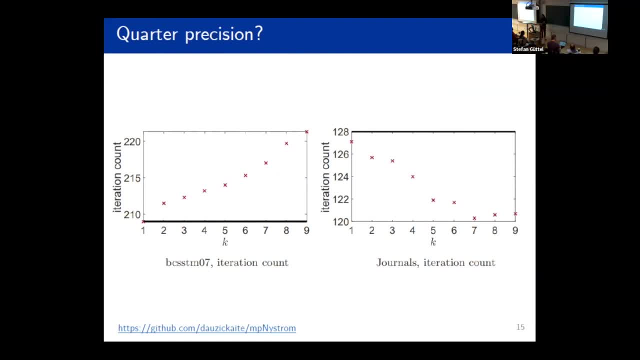 i'll say for our, for the problems we tried. it didn't really work very well. okay, it doesn't really give you very much um. so here this is the same matrix i was using before this, bc sstm07 um. actually, here, when we use quarter precision, and this is the variant with, with uh, three significant 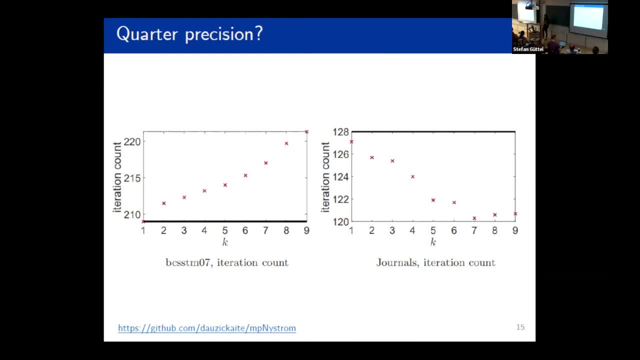 bits. um, the, the iteration count goes up, all right, so it's a terrible preconditioner. um, we did find some one example where the, the iteration count does go down, so it's the the preconditioner is doing something, but if you look at the, the y-axis here, it's not doing very much. okay, um, so is is. 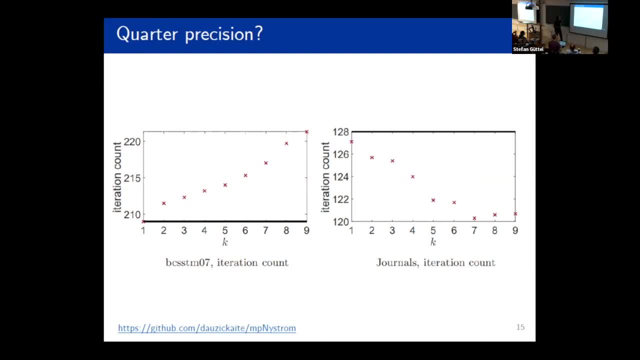 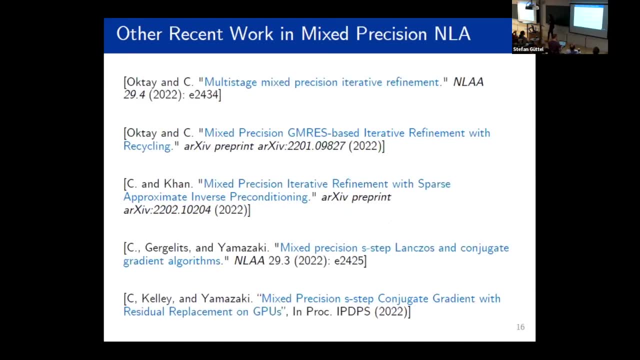 there a use for quarter precision? i, i believe that there is. maybe we have to. we have to do something more clever here to get to work for us at our own. okay, all right, and so just to self-advertise a little bit, uh, while i have your attention, so i've um nick. nick was really, uh, inspiring for me, um, and. 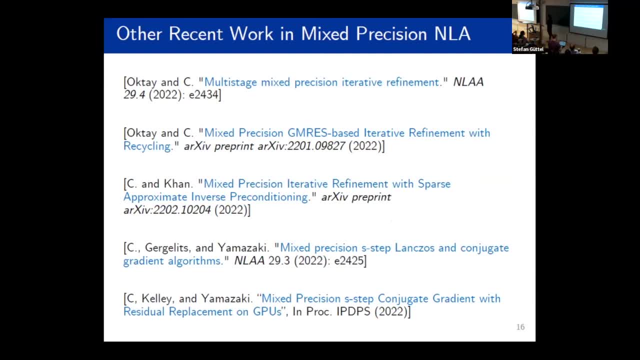 and i've done a lot of work on, on mixed precision, uh, numerical linear algebra since then. um so this is a- you know, a lot of work for me and also for for my phd students. um so we've worked on multi-stage, a mixed precision iterative.